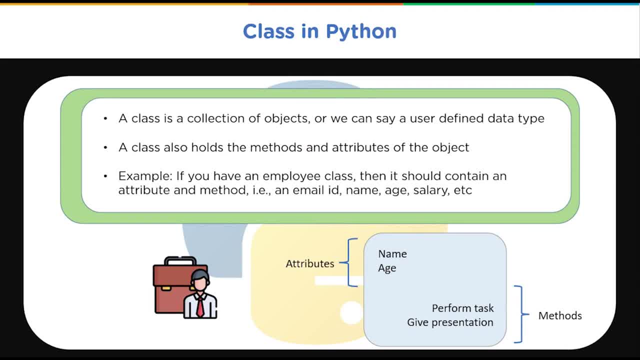 and abstraction. Now, what is a class? Class is nothing but a collection of objects, or we can say a user-defined data type, right? So basically, it's a complex data type which has a collection of objects, and within the objects you have primitive data types like 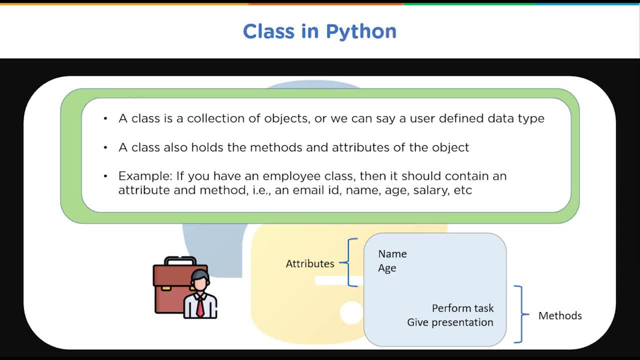 int, string, float, etc. So a class also holds the methods, the functions which basically perform operations on these objects, right, and also it also holds on to the attributes of the objects. So let's see with an example: right, So if you have an employee class, then 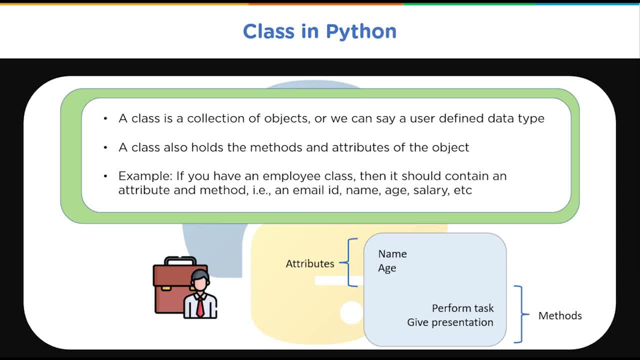 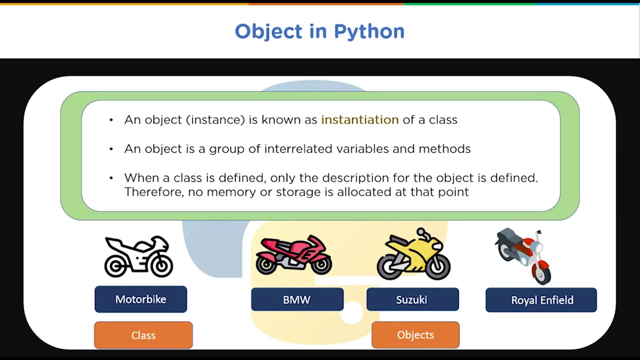 it would contain attributes and methods, such as email id, name, age, salary. These are the attributes. and on the methods, like you know, perform tasks, give presentation, increase salary, etc. etc. These are will be the methods. Now let's talk about what are objects in Python Now, object is known as instantiation of a 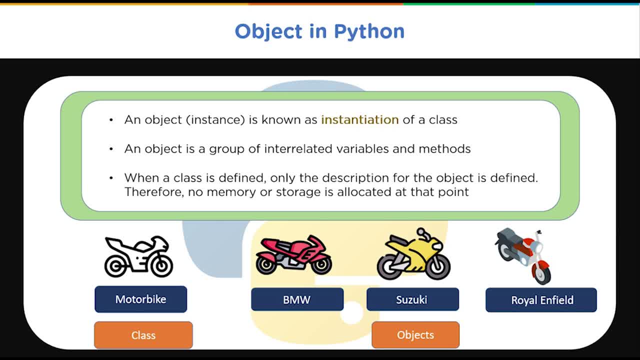 class right. An object is a group of interrelated variables and methods. So when a class is defined, only the description for the object is defined. Therefore no memory or storage is allocated at that point. So for example, if you see in this motorbike is a class, but 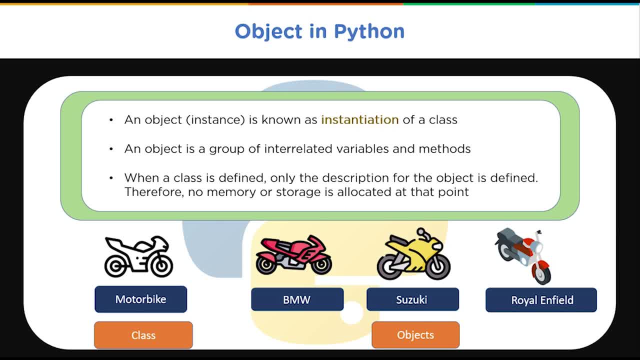 the different objects of the class are different kind of bikes by different brands like BMW, Suzuki, Royal Enfield. So they all have inherited the attributes of the class motorbike and then on top of it, Variables, additional variables and methods on top of it to enhance the motorbike and make it look different or function differently. 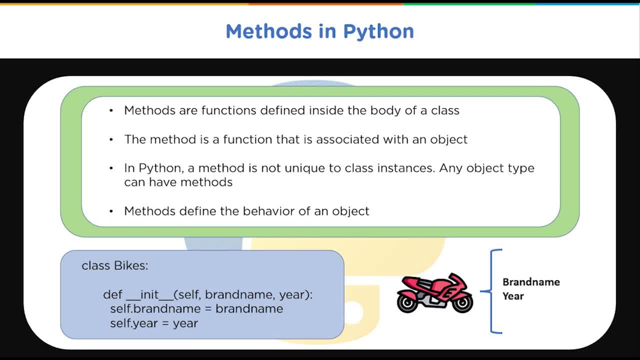 Now, what are methods? in Python, Methods are functions defined inside the body of a class right. So basically, methods are something which you perform on attributes of a class right. Method is a function that is associated with an object, So you create an object of a class and on that object then you can execute those functions. 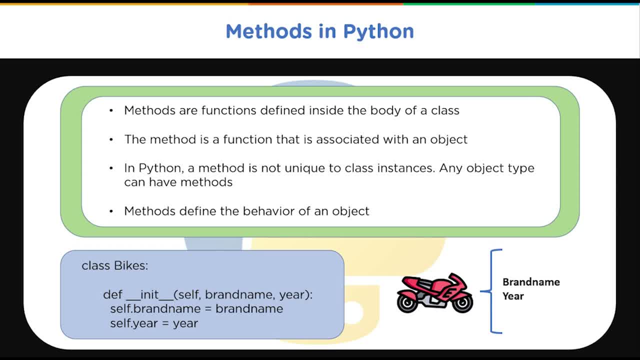 In Python. a method is not unique to class instances. Any object type can have methods And the methods define the body, The behavior of an object. So that's why a BMW motorbike will be different from Royal Enfield: because the behavior is different. 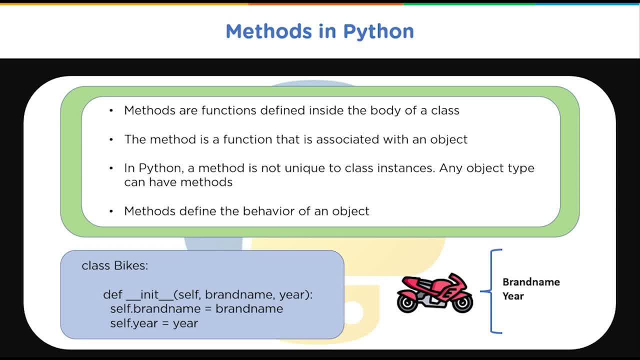 The methods are different. So if you see the example over here, you have a class bike And in that there is an init function which will get invoked when you initialize the object of class bike, And then you can set the brand name and the year of manufacturing for that particular object. 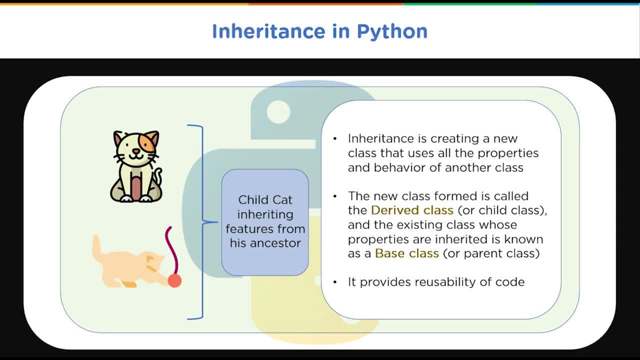 Now inheritance. what is inheritance? Inheritance is something which you derive from a parent. So inheritance is like creating a new class that uses all the properties and behavior of another class. Now the new class is called the derived class or the child class. 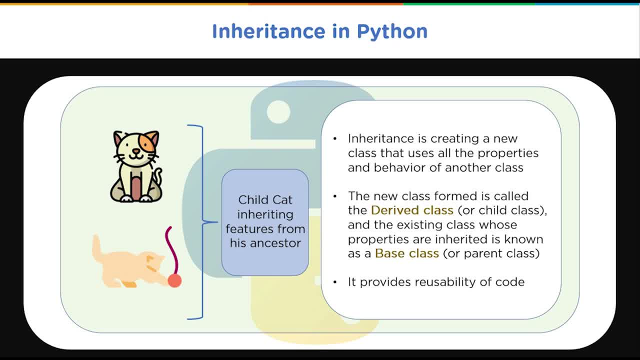 And the existing class whose properties are inherited is known as a base class or parent class. It provides and the basic use functionality. the usage of inheritance is that reusability of code. So if anything is defined in the parent class then you don't need to rewrite that particular code in the child. 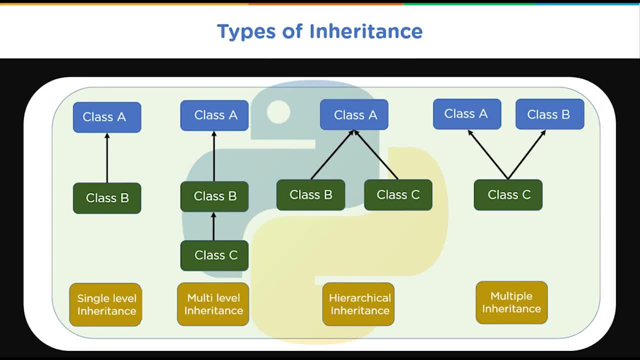 You can just inherit it. So, as I mentioned, let's take a look at the different types of inheritance which are available. You have single level, in which only one child is inheriting the properties and the attributes. Then you have multi-level, in which first child has inherited from the class A, class B has inherited. 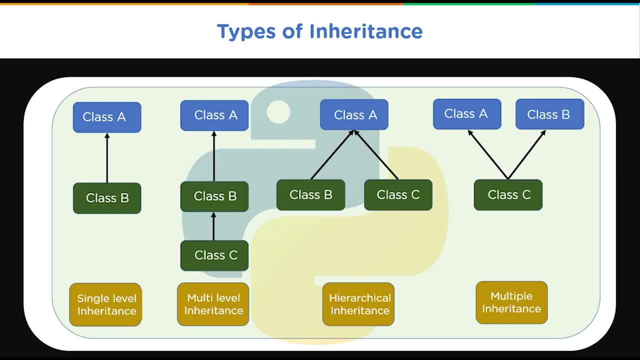 And then you have another class C which is inheriting from class B. So this is an example of multi-level And we will be supporting all these concepts with an example in our Python notebook. Then there is hierarchical. Then there are two different classes which are inheriting from a single class. 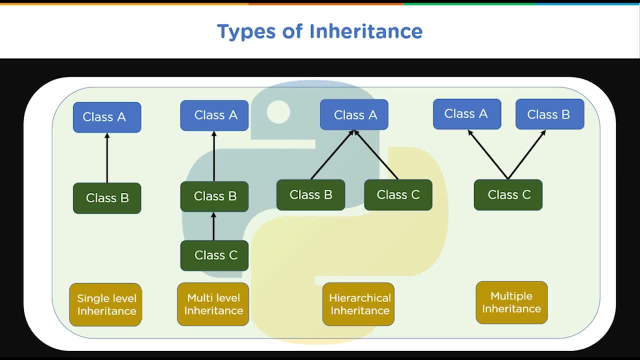 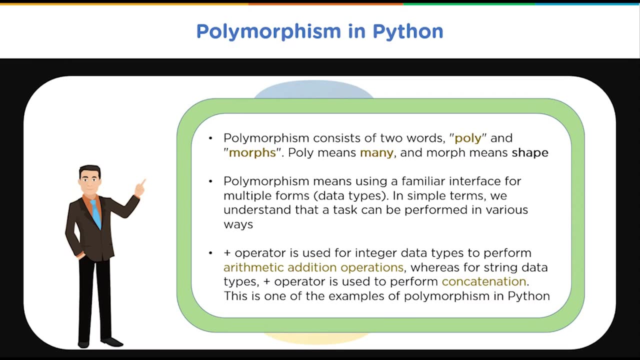 And then Multiple inheritance, that single class is inheriting from two different parents. So these are different set varieties of inheritance basis. What is the demand? What is the business requirement you can define Now, what is polymorphism? Polymorphism in Python. 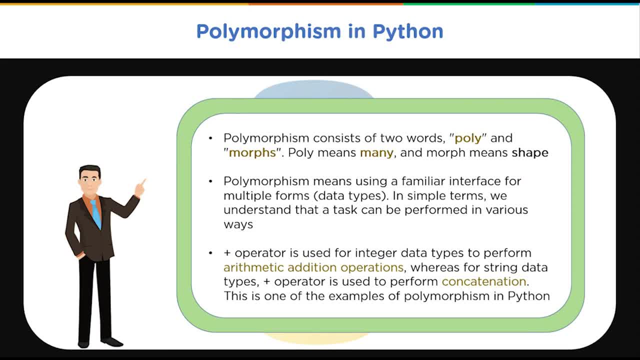 What does it mean? Polymorphism consists of two words: poly and morphs. Poly means many and morph means shape. So basically, It means a many shapes. So it is. It means using a familiar interface for multiple forms, right? 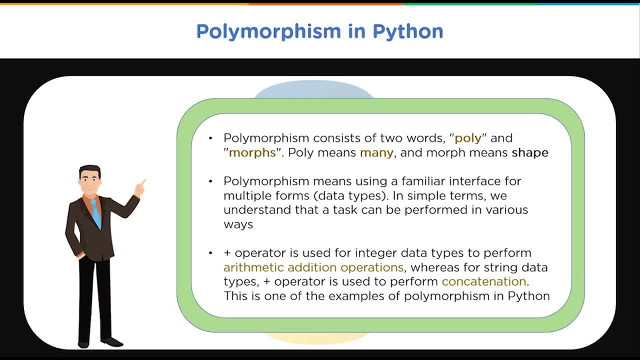 So you can use a single name of the method and which can perform different behavior based on the object in which it is invoked. So, in simple terms, we understand that a task can be performed in various ways. Let's support it with an example. 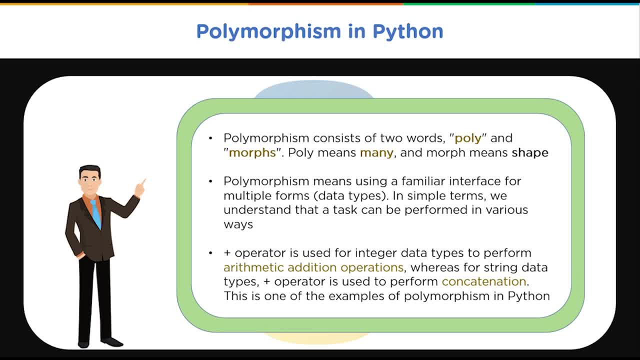 Like you have a plus operator. Now the plus operator can be used for integer data types to perform arithmetic operations, Whereas when you use plus operator to in string data types, it can be used for concatenation. So it's a very typical example. 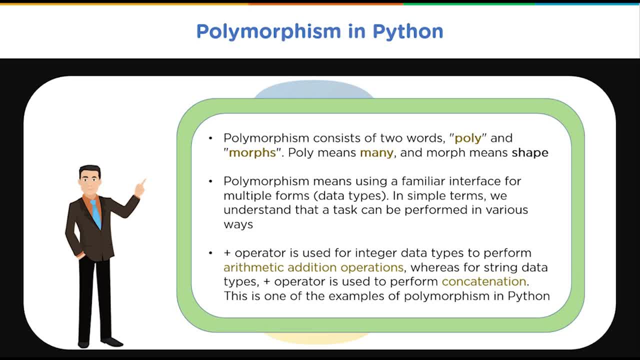 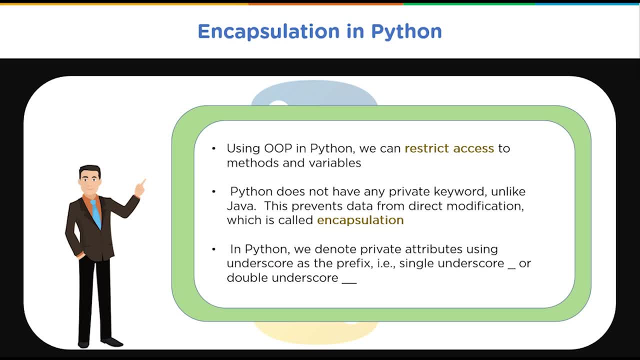 Very good example in terms of how an thing Same operator can behave differently. basis: What data types are being used. now let's talk about encapsulation. using oops in python, we can restrict access to methods and variable. so basically, in in python you can, you can create something like as private variables: 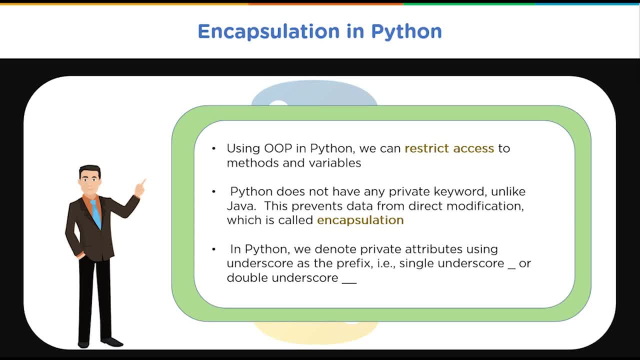 but of course you can't use a private keyword, unlike java. so in in python we use underscore or double underscore in order to define private attributes. so basically, these attributes can be only used within the class and cannot be exposed outside a particular class. so we will see this with an example. 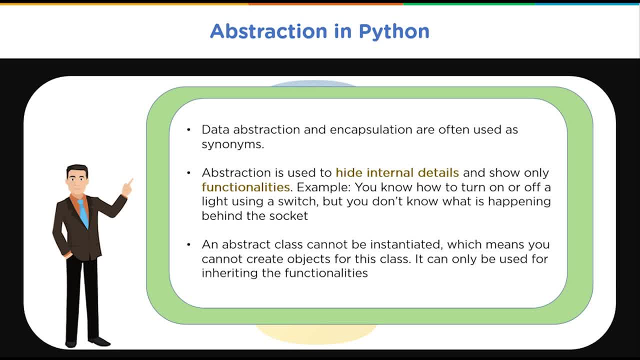 now, what is abstraction? data, abstraction, encapsulation are often used as synonyms. abstraction is used to hide internal details and show only functionalities. for example, you know how to turn on or off a light using a switch, but you don't know what is happening behind socket. similarly, an abstract class cannot be. 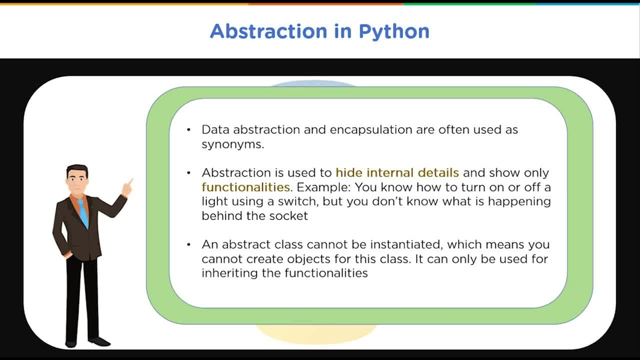 instantiated, which means you cannot create objects for this class. you can only define the methods which have to be implemented by the classes which are inheriting the abstract class. so basically, abstract class is a class which is not a class, which is not a class which is not a class. 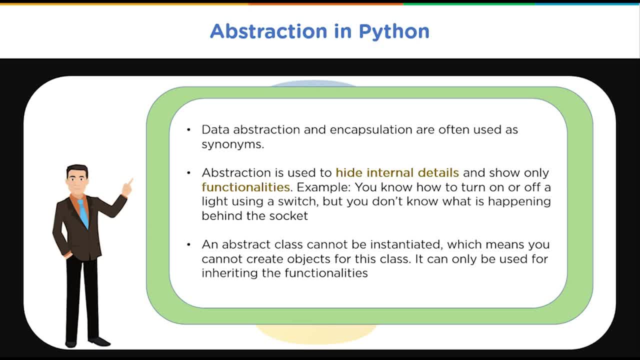 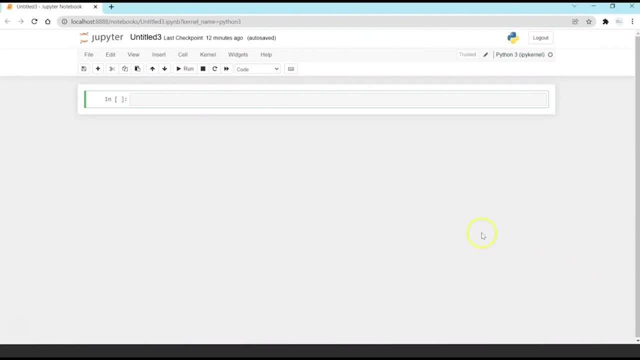 like do the abstract class provide only the method signatures and rest the other functionalities and the implementation has to be done by the child classes. so let's now move to the, our jupyter notebook, and we will start performing certain examples. now, as we are saying, like python has objects, so let's create a. 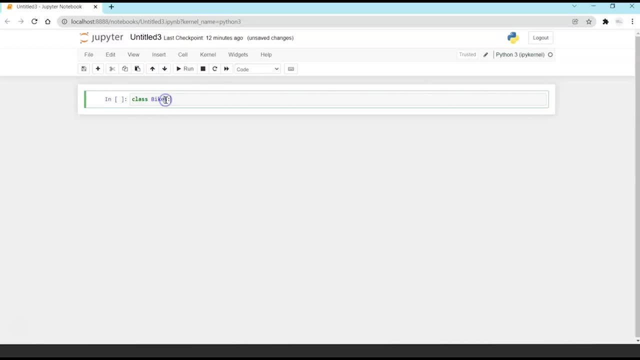 object. we will create a class bikes over here and within the class we will define the init method and in the init we will instantiate two variables: brand name, and here now we will create and object of bike, which we will real, we are calling as BMW, and another we will create an object called Ducati. so what we are doing in 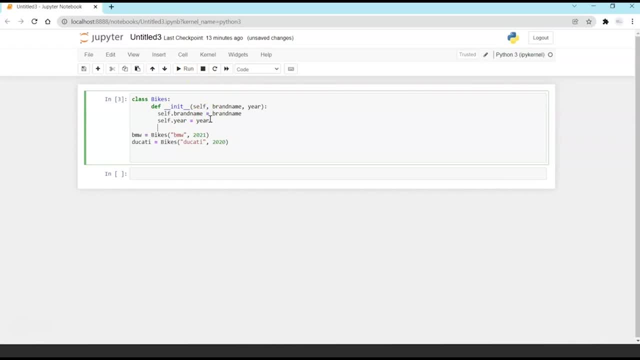 this to scenarios is that we are just instantiating the byte of bike object with variable BMW and Ducati. we are instantiating now let's print the year and manufacturing year, the brand name and the year for BMW and for Ducati and let's see right. so what we have done is we have created an object for bikes, one. 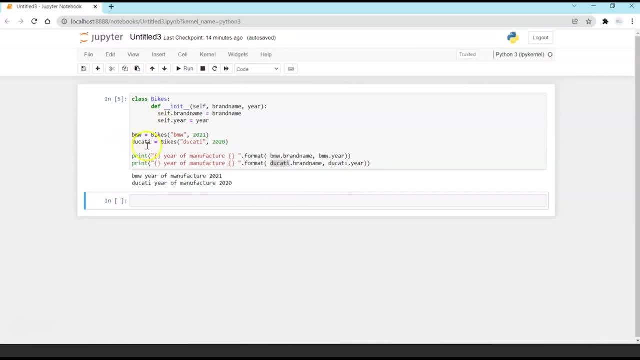 we are calling BMW and one we are calling Ducati, and how we are differentiating between these two bikes is basis, the brand name and the year of manufacturing. now let's take a look at the example of methods. I'm gonna rewrite my init method and now I am creating an function: a method of top speed and a function of. 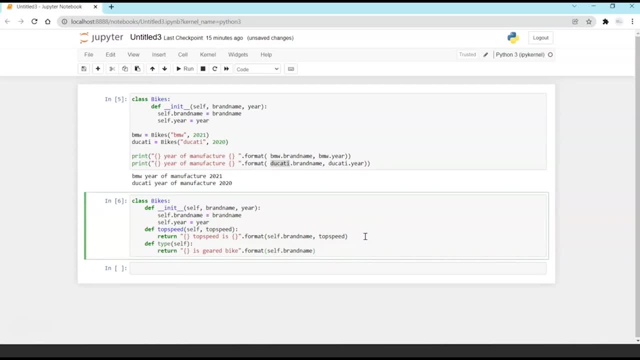 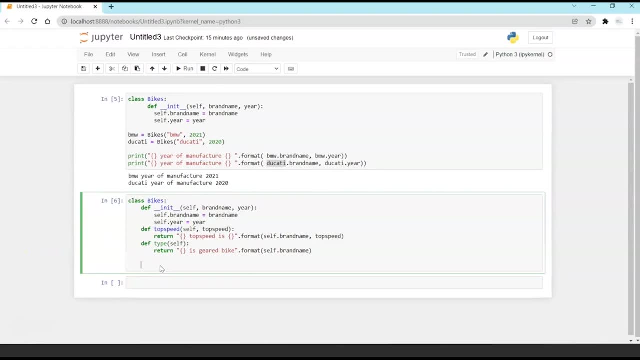 type. I'm gonna create an object of bike. now this method, this object bike, can invoke methods top speed and type, because they belong to the same class bikes. so initially, when I created my object bikes, I am instantiating with BMW and the year, and then I'm making a call to the method top speed and then I'm making a call to the 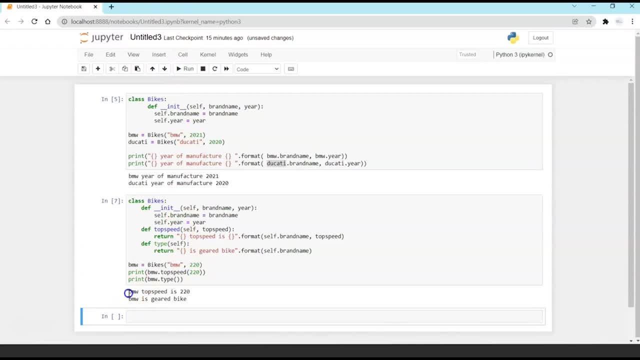 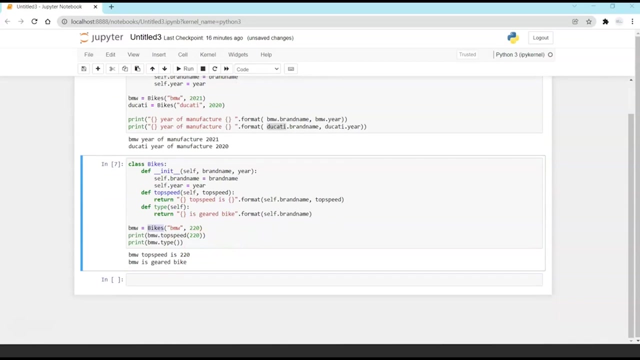 method, type and printing. so basically I'm printing the output of the function top speed and output of the function BMW. form the object: BMW, which is of class bikes. now let's take a look at the network of the bike here. let's take a look at the layout as an example of 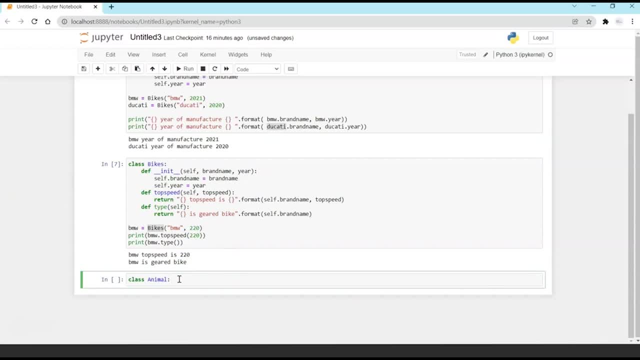 the bike platform we can pick bike- única seoun. there is no bicycle here. to show what's happening first let me do a little 長 grams here and arma Pala is the amount of quality in which the bike will work. but the price of bike is only around six pesos. now the price of bike. 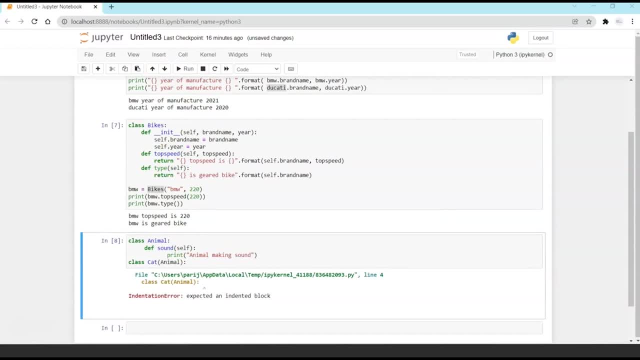 choice. we need the tourists. let me just put a method over here. yes, the indentation. okay. so now i have object: parent class animal, child class cat which has inherited animal, and the parent class method is sound and the child class method is meow. so now i'll create an object. 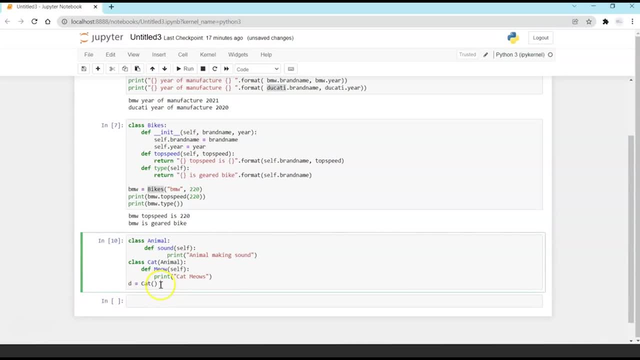 called cat and with this object i'll be able to invoke both child class method and the parent class method and, as you can see, uh, the child class has inherited both uh, parent and child class function functions methods. now let's take a look at multi-level inheritance example. i'll start off. 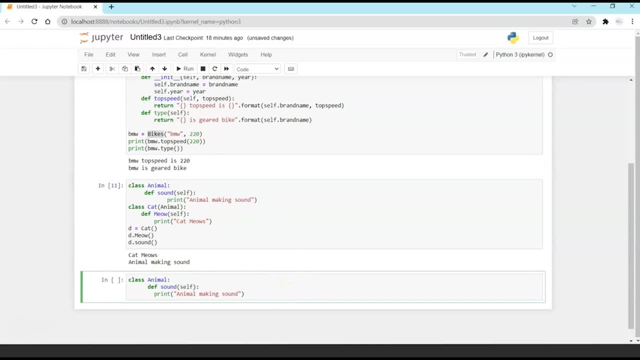 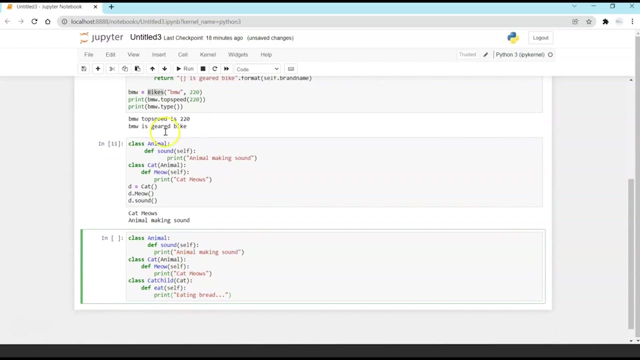 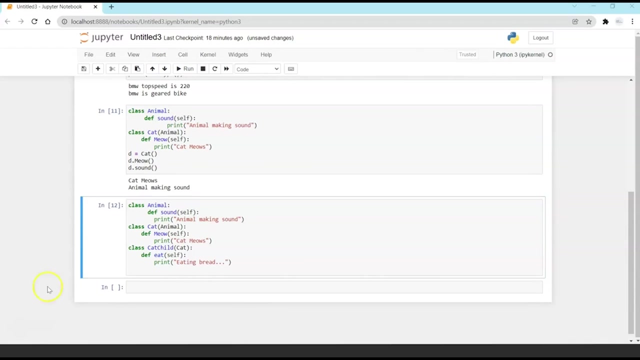 with creating exactly the same parent class called animal. then i'm i've already created another class. i'll create same child class, cat, and now i'll create another class which will inherit cat class. so cat has inherited animal and cat child has inherited cat. let's validate its syntax. and similarly, now i'll create an object for cat child. 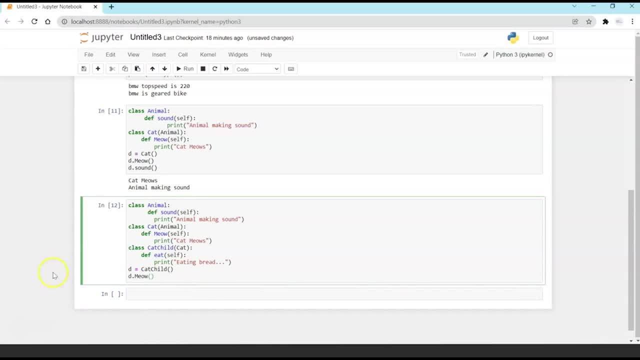 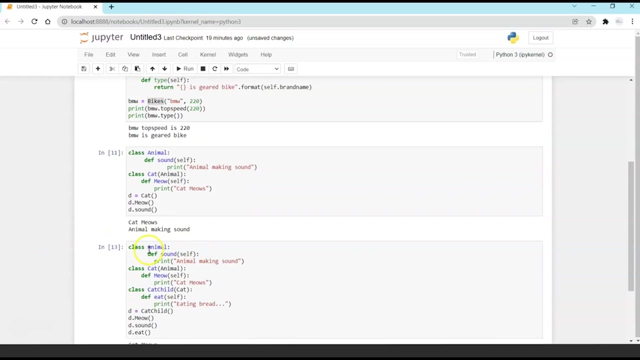 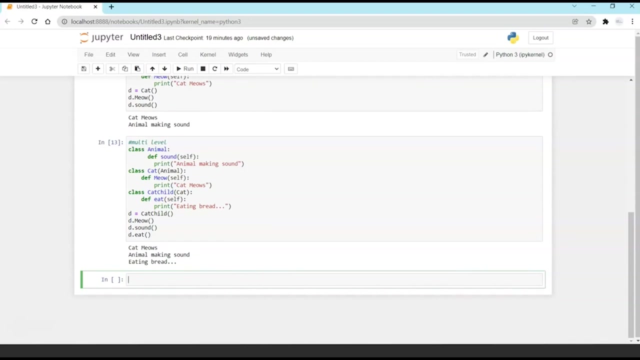 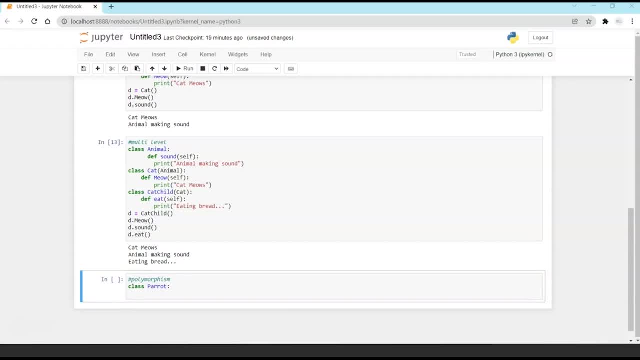 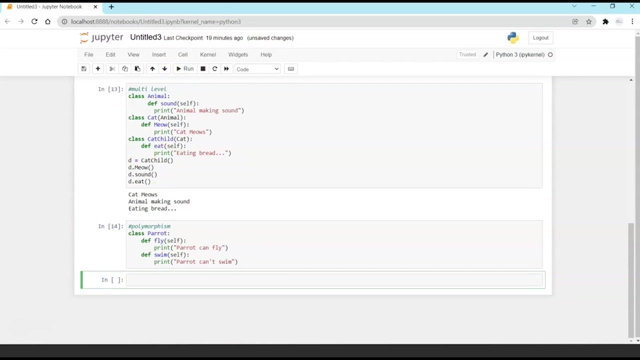 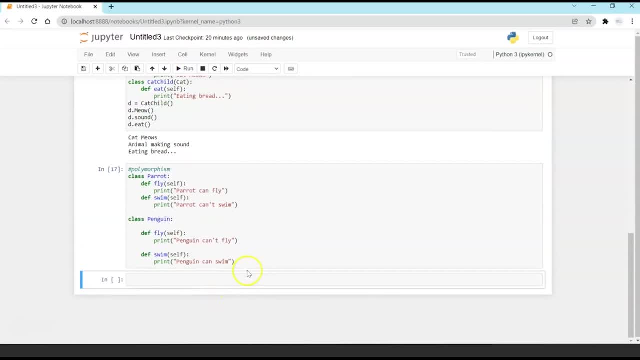 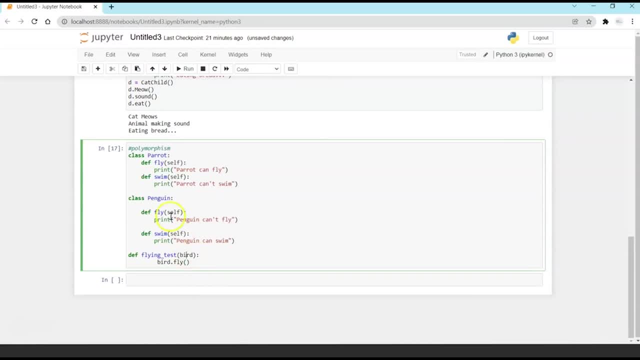 instance of the particular object, bird it- the corresponding method will get invoked. so let's see in the method flying test: whatever instance of the bird object will be, the corresponding of method will be called. so now let's create a object of parrot class and then let's create a object of penguin class. 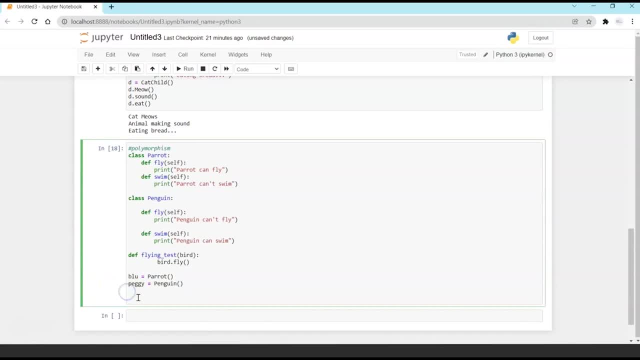 now in my flying test method, first I'll send a object of instance- parrot, and then I'll send the object of instance penguin. so now, basis the instance type. when this bird dot fly method will be called, it will be called basis the instance. so in the first case, the parrot, it will call this. 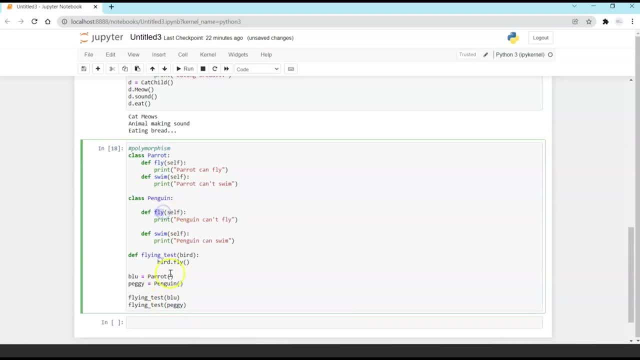 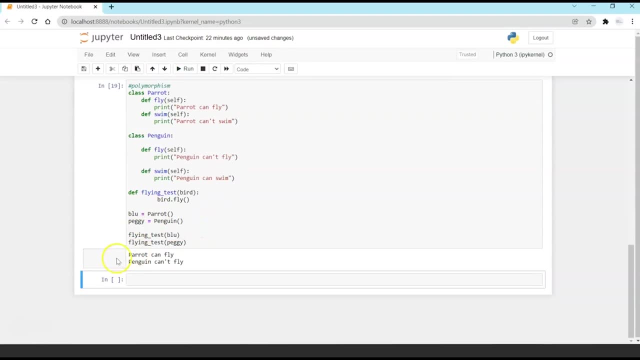 method and in case of penguin, it will call this method fly. so please note what is the output. the output is a parrot can fly, but a penguin cannot fly, and it has been decided by the Python at the runtime that which particular method to be invoked basis the instance. so it's a very important concept. 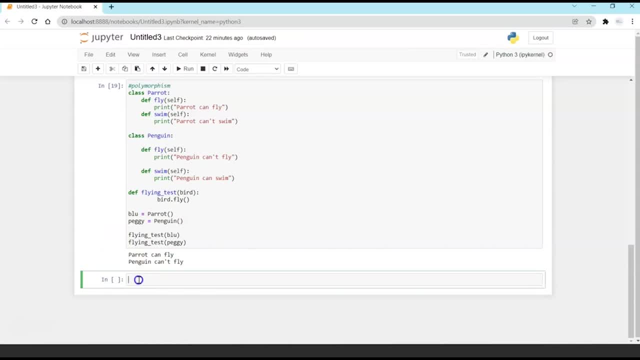 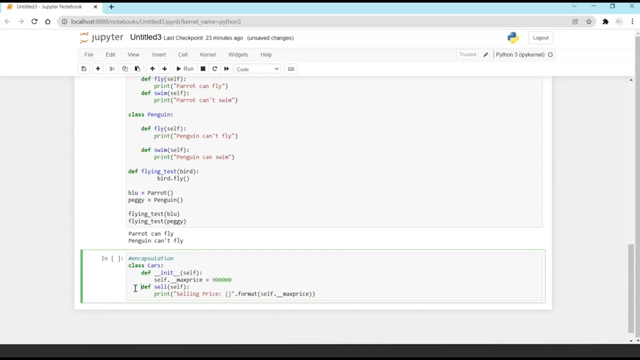 now let's take an example of encapsulation. I'll make a class, cars define its init method. now, within that init method, I have created a private variable with underscore, underscore max price, and given a value of nine lakh. and now I am creating another function called cell, and in that I am printing the 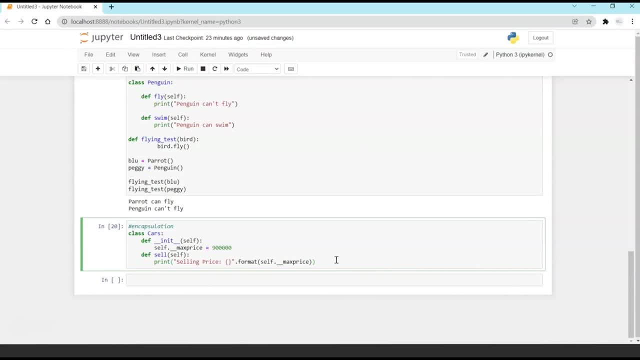 max price. and then I am creating another function in which I am modifying the private variable set max price. so I will pass any value in the set max price and it will replace the max price which I have set during the initialization at this point. now let's create an object of class cars and see if I sell this then. 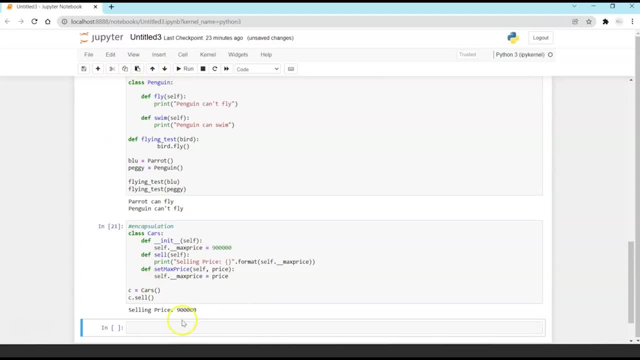 the selling price is nine lakh. what I have done is I have created a private variable, but I had any at the set at the time of initialization. now what I am trying to do is I am trying to modify a private variable directly- see underscore- underscore: max price- and I want to check if I am trying to create a, modify a. 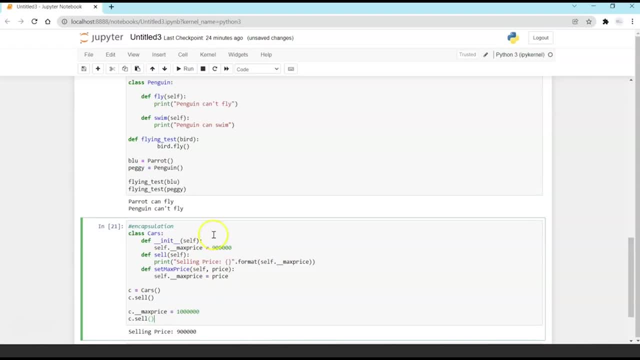 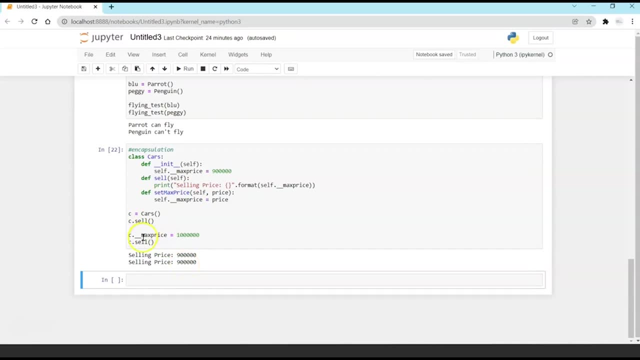 private variable, will it still show me nine lakh or ten lakh value? and it's still showing me the nine lakh value. it means that I can't directly modify a private variable. I can only modify it if I access it through a method which is set max price. in this now I am setting the max price to thousand. and now if I print, 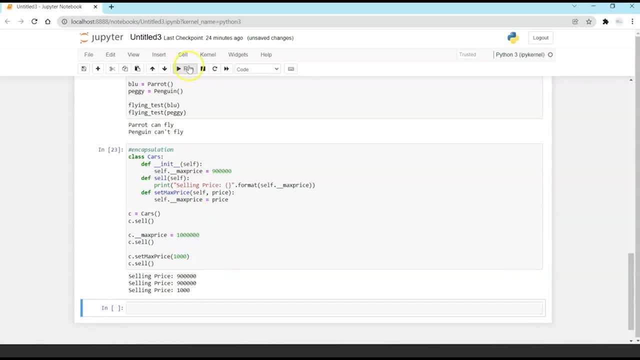 what is my max price? it will print as thousand. so this is the concept of encapsulation. you have a private variable which is accessible within only the methods of the class. you can't access it directly. now let's take a look at hierarchical inheritance. I'll create a class employee. 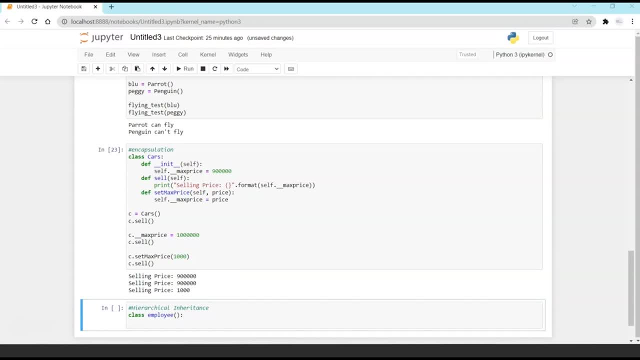 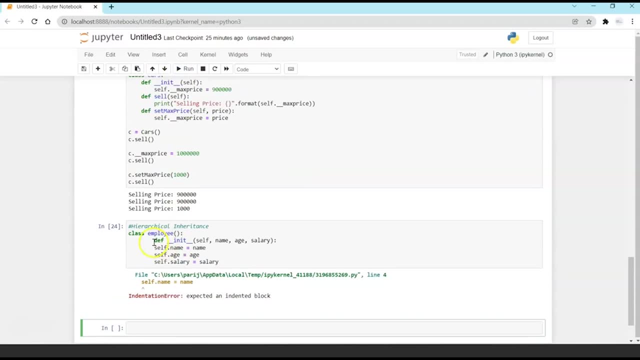 and Pln method, create an inert method. within that you have three variables, Ged of three line: name, age and salary. So an employee which has name, age and salary. now I'm going to create a class, child class called child employee, one which has inherited from employee and child employee two. 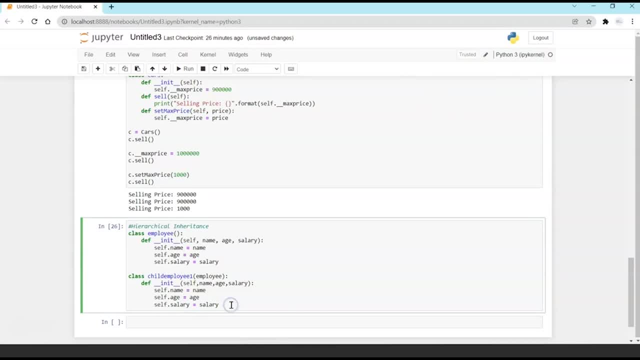 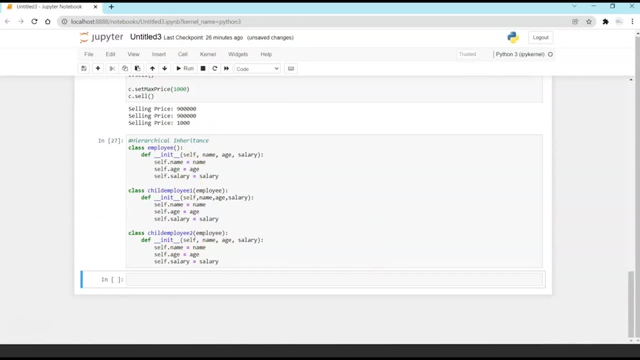 deed: name, age and salary. Now I'm gonna create a class, child class- called child employee, one which has inherited from employee and child employee to the child employee2, which is also inherited from employee. so what I am going to do is I am going to create a object per child class and print. 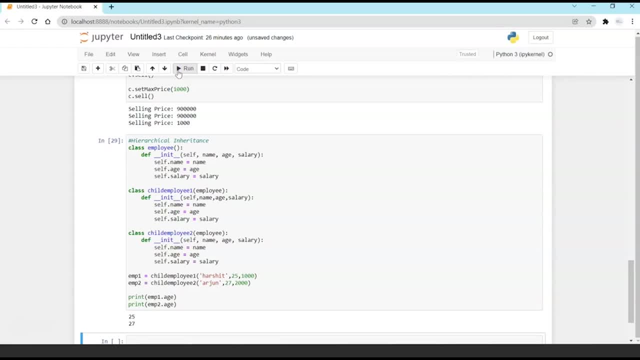 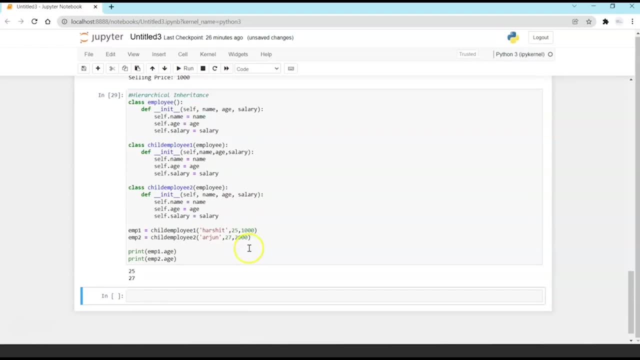 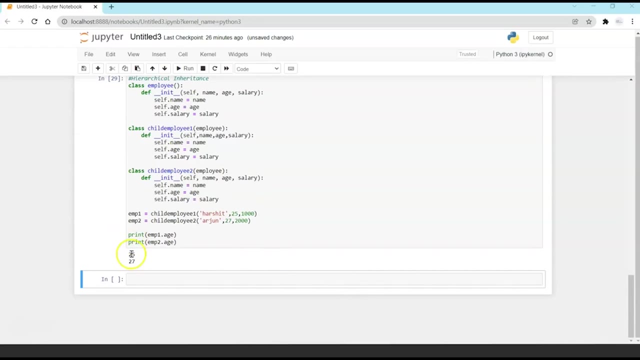 so this is a typical example in which you have two child classes which have inherited from the single parent- hierarchical inheritance. now let's take a look at our last concept, which is abstraction. so now I'll create a class car and define a method mileage, but I am not giving any definition.